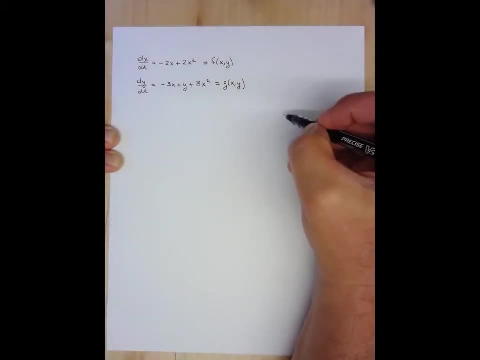 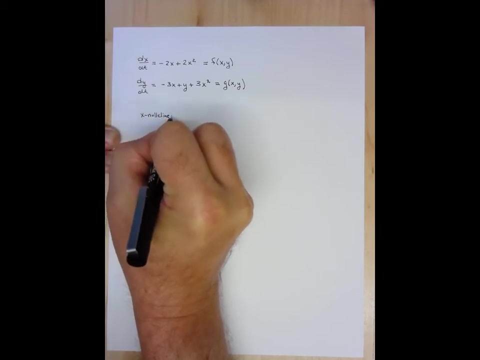 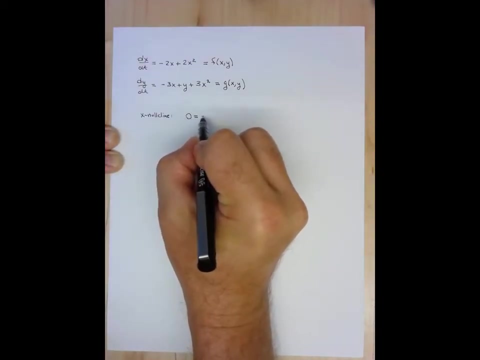 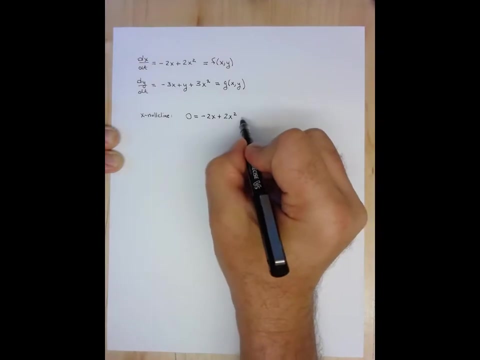 begin the phase plane analysis, why don't we first see if we can easily determine the nullclines of this system? So the x nullcline will be determined by setting the left hand side of the first differential equation to zero. So that's zero equals minus 2x plus 2x squared. This can be factored. We can also. 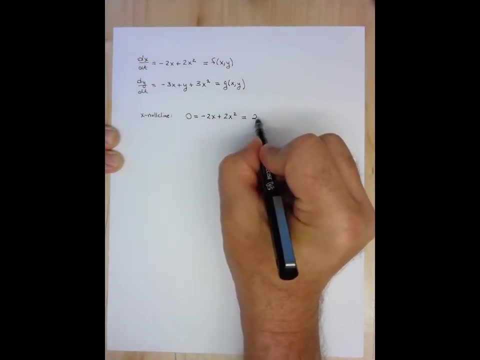 pull out a 2x, So this is equal to 2x times negative 1 plus x, which is 2x times x minus 1.. So the x nullclines are all the points satisfying. zero equals 2x times quantity x minus 1, which is: 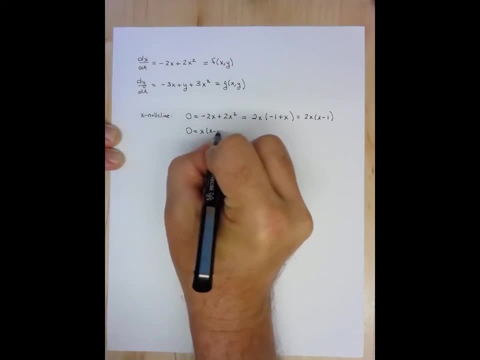 the same as zero equals x, So we can pull out a 2x. So this is equal to 2x times negative 1 plus x, which is 2x times x minus 1, just dividing both sides by 2.. So the x nullcline is given by x being. 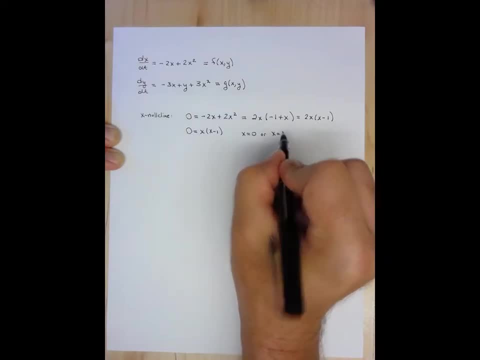 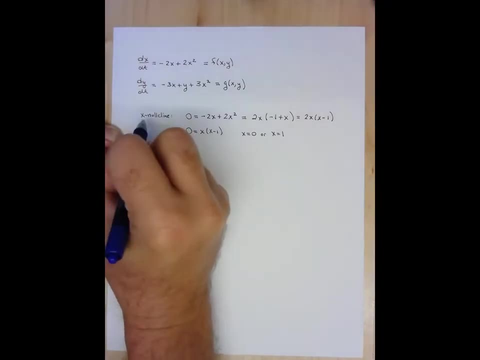 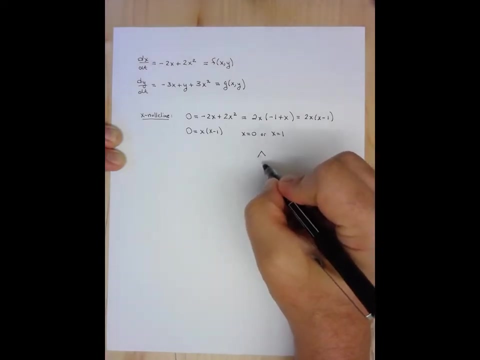 equal to zero, or x being equal to 1.. So the x nullcline will have two branches and they'll both be vertical lines. So let me see if I can sketch that for you. This is the y-axis And the x-axis, And if this is the 0.1, then the x nullcline, if I sketch it in blue, will be this: 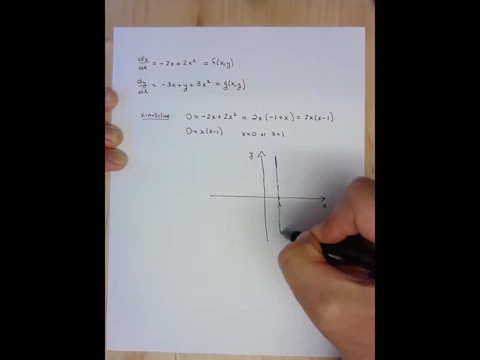 vertical line going through x equals 1.. Result is: a vertical line going through x equals 0.. So now we have a vertical line going through x equals 0.. So now we have a vertical line going through x equals 0.. Note that the x nullcline in blue here it's not continuous, It's not contiguous, There's actually 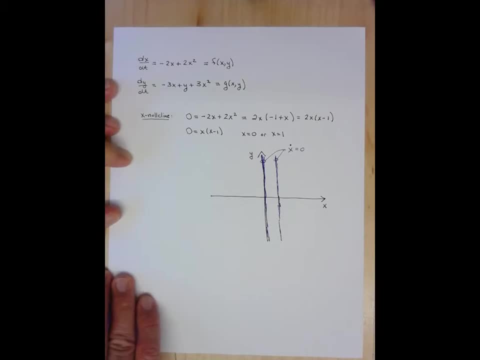 two lines where the rate of change of x is going to be equal to 0 on any of the points on either of those two lines. Now for the y nullcline. The condition is setting the y nullcline, the rate of change of y, equal to 0. And so that's 0 equals. 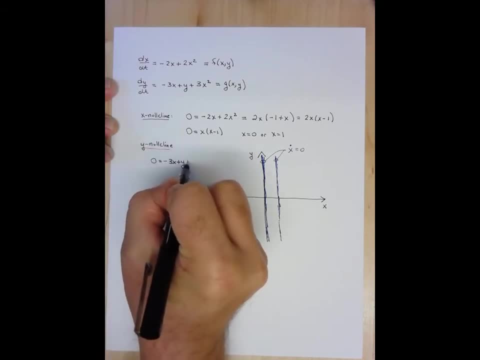 minus 3x plus y plus 3x squared. And it looks like if we bring everything but y over to the left, we'll have 3x plus 3x squared, And it looks like if we bring everything but y over to the left, we'll have 3x plus 3x squared. 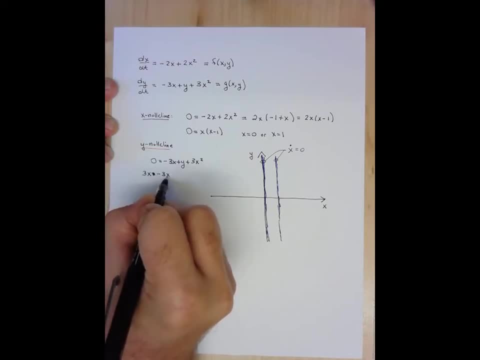 Minus 3x, squared is equal to y, And then we can sort of flip this around and say y equals, and then we'll factor out the 3x. We'll go 3x times 1 minus x. So this is the equation. 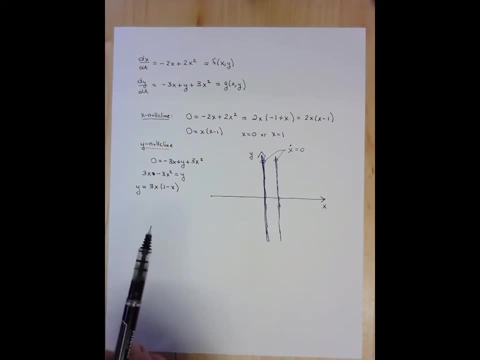 for the y-nalcline and it will be a concave down parabola. I can see that because of the negative sign in front of the x squared term, and this concave down parabola will intersect the horizontal axis at 0 and 1.. 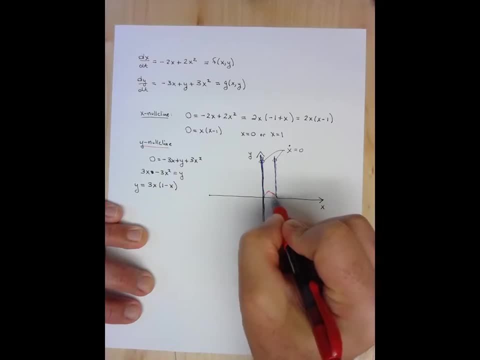 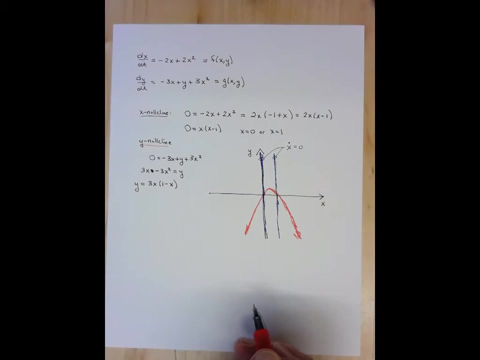 So I'll attempt to sketch a concave down parabola that intersects the horizontal axis at 0 and 1.. All right, so this is the equation for the y-nalcline. So I'll attempt to sketch a concave down parabola that intersects the horizontal axis at 0 and 1.. 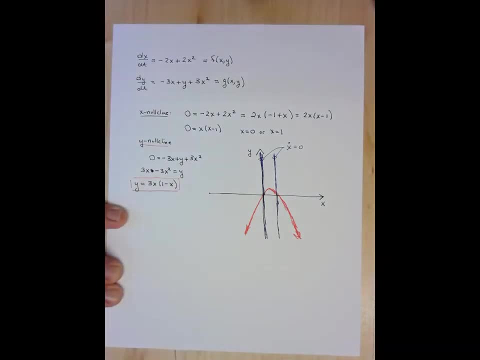 All right. so this is the equation for the y-nalcline. Any set of points x and y that satisfy that equation will be on the red line. and this is the equation, or equations, for the x-nalcline here. So we know now that certainly that there's two steady states. 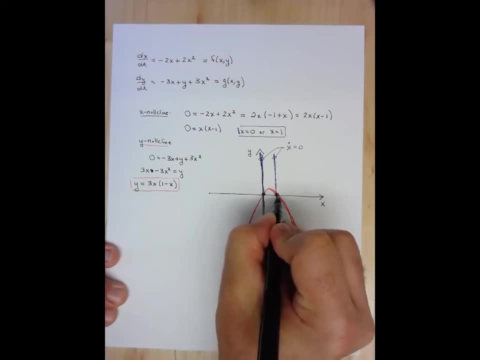 There's two points in the plane where the x and the y-nalclines actually meet. So when we consider the steady states, that's quite a lot of points in the plane. So when we consider the steady states, that's quite a lot of points in the plane. 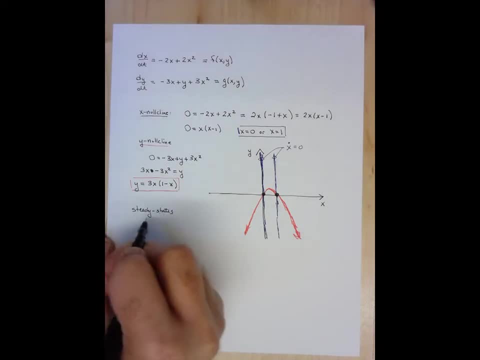 easy to see now. So one steady state is both x and y being equal to 0, and that's this one. And there's another steady state, which is x and y being equal to 1 for x and 0 for y, and that's to the right. 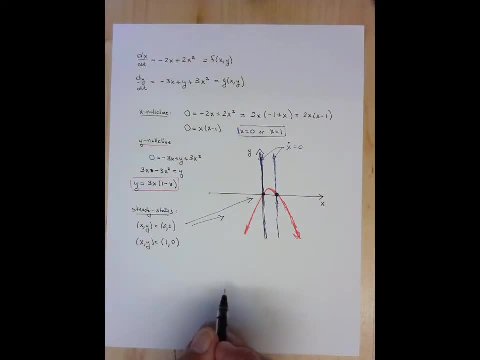 So what else can we do? Well, in addition to determining that these steady states occur at the particular values of x and y that we have indicated, we can also analyze the stability of those two steady states. I think, in this case, I'll do that even before I sketch any. 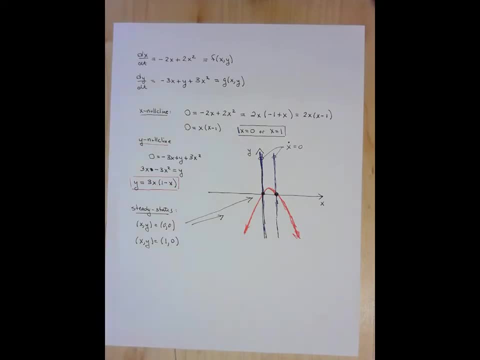 flow on the phase plane. So remember, in order to do that, we're going to calculate something called the Jacobian. So this is now linear stability analysis. So what is the Jacobian of this system? It's a function of x and y, potentially, and it's the. 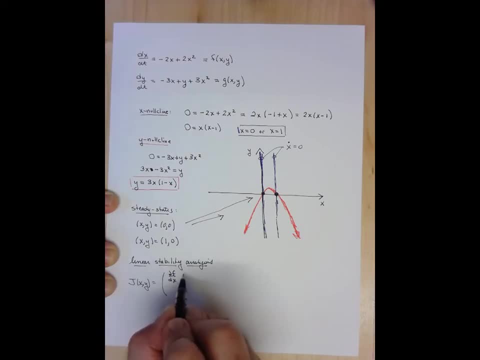 partial derivative of the first equation with respect to the first variable and then the partial derivative of the first equation with respect to the second variable. This element is the partial derivative of the second equation with respect to the first variable and this element is the partial derivative of the second. 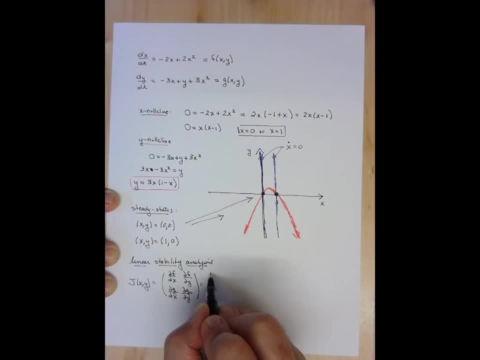 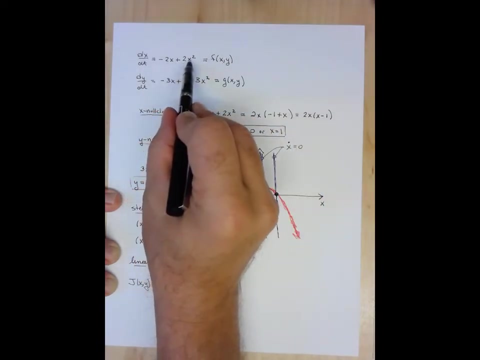 equation with respect to the second variable And if we calculate those partial derivatives we'll get the Jacobian matrix Up here. we see that f of xy is minus 2x plus 2x squared. So the derivative of that function with respect to x is: 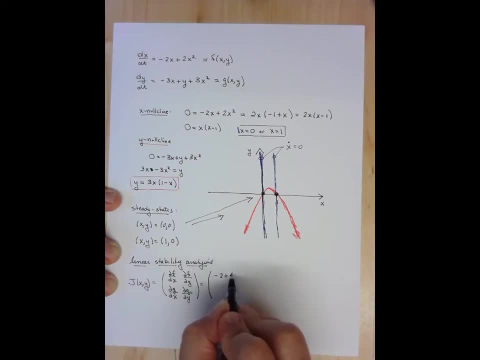 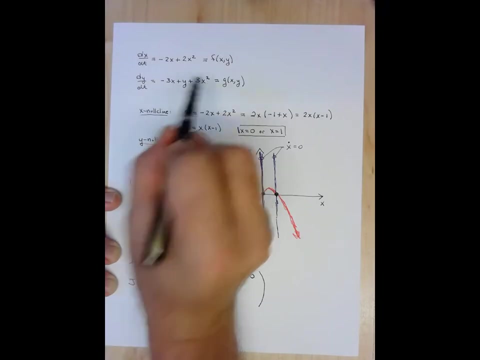 minus 2 plus 4x. The derivative of that function with respect to y is 0.. Now g of x is minus 3x plus y plus 3x squared, The derivative of that function with respect to x is minus 3.. 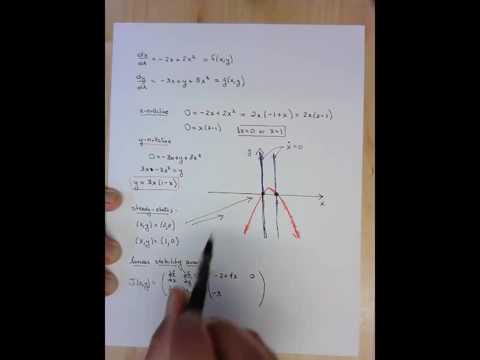 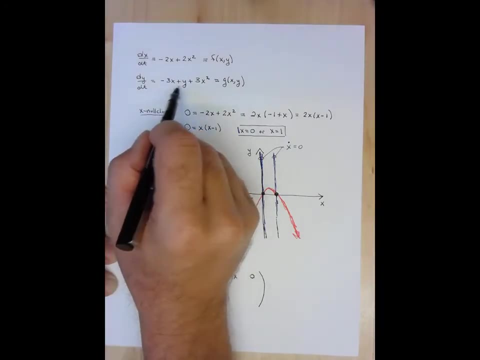 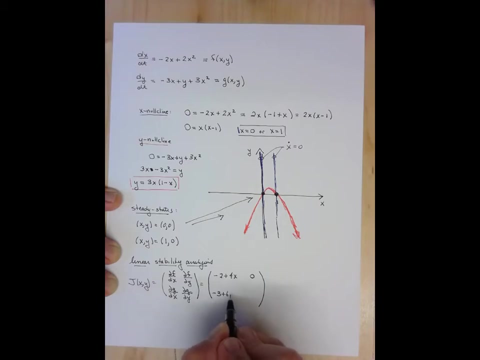 The partial derivative of g, the function g of xy with respect to x. when we take the derivative of the y here, what we're thinking of? y as a constant, and so we'll get 0.. And then the 3x squared term will yield 6x. 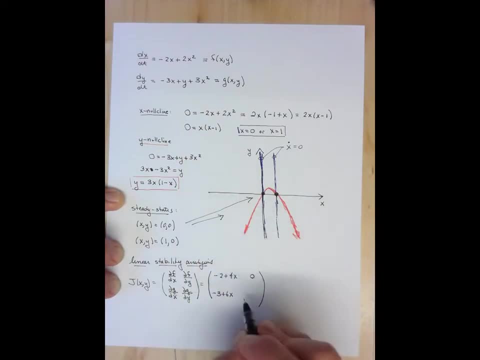 The partial derivative of g with respect to y is just positive, 1.. And now to do linear stability analysis, we need to evaluate this Jacobian at the two steady states. So the Jacobian At the first steady state, 0,, 0, is the constant coefficient. 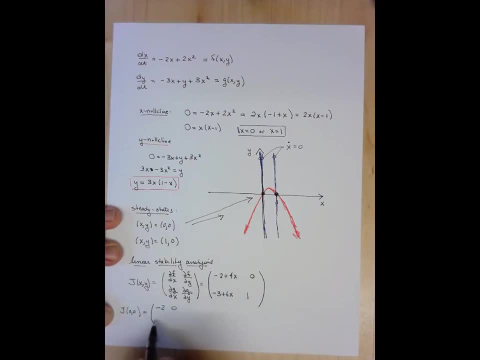 matrix minus 2, 0, and minus 3, 1.. And the Jacobian matrix at the steady state, 1, 0, is equal to minus 2 plus 4 times 1. So that's plus 2.. 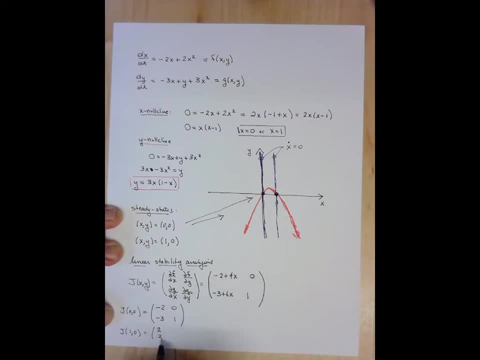 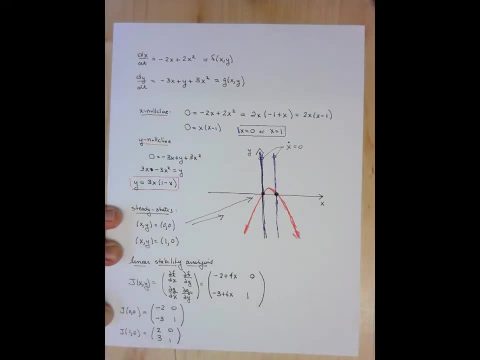 We'll still have 0 and 1 over here. So those are our two Jacobian matrices. And to continue the linear stability analysis, let's consider the trace and the determinant of these two matrices. So the trace of this Jacobian matrix is negative 1.. 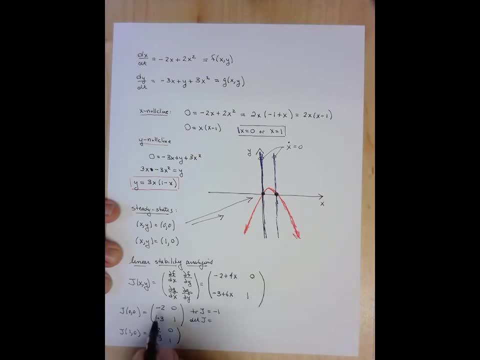 And the determinant in this case is minus 2 times 1 minus 0 times negative 3. So that's simply minus 2.. In this case, the trace is 2 plus 1, or 3. And the determinant is 2 times 1 minus 0 times 3,. 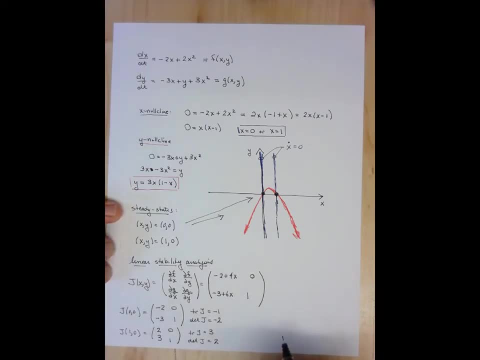 or positive 2.. So we can see here that neither of these two matrices of these equilibria will be stable, Because the condition for stability is that the trace is negative and the determinant is positive, And neither of these two satisfy that, So both are unstable. 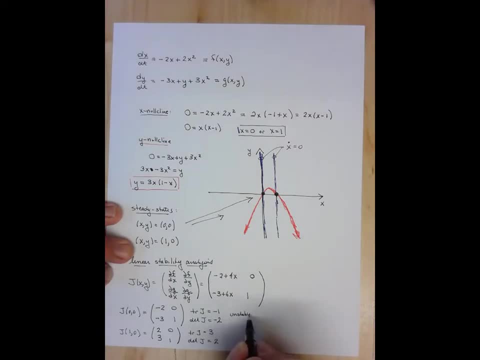 And neither of these ones do, But all of them are stable. So the only way we'll be able to deal with that is if we can just read this derival line to replace theophobia variation. So now let's see if we can get a little bit more information. 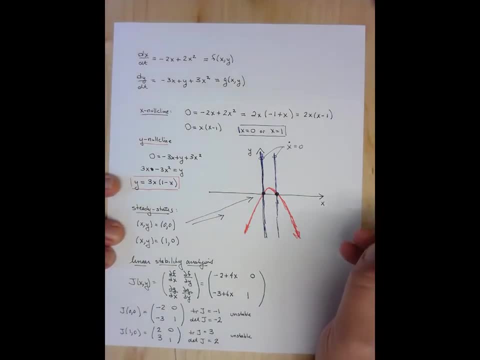 about the solutions in the phase plane, And this is really interesting. We have a solution H star and v theta and theta minus 1.. A solution crossing an x nullclient can only do so in the vertical direction because the rate of change of x has to be zero. 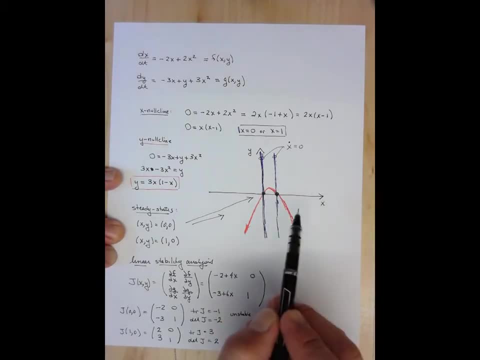 So it's pretty clear that both of these vertical nullclines for x are separatrices. The solutions are not going to be able to move from one side of those lines to another Right, Because if you were on one of the x nullclines, the rate of change of x is zero, so you can't move to the left or to the right. 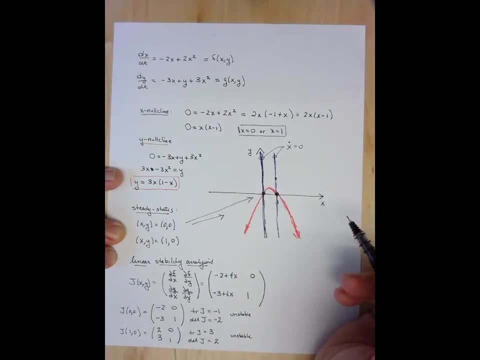 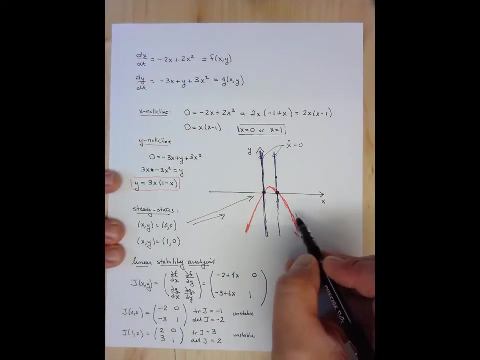 You can only move up or down. So in fact you can actually see that these lines will be trajectories of solutions that are actually following these nullclines. We'll see that in a minute. Let's see For the y nullcline, the rate of change of y is zero and if the y nullcline is going to be crossed, we're going to have to do so in a horizontal way. 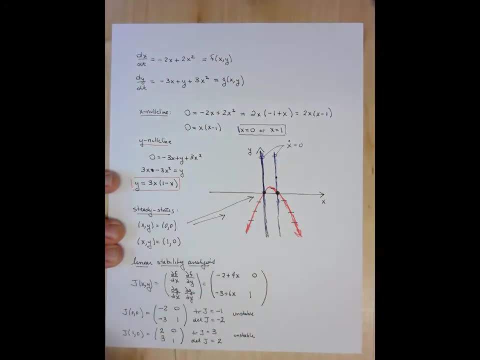 Right, Because moving horizontally is the rate of change of y being zero but x being non-zero. Now can we figure out the actual direction that things would be moving in the various quadrants. That's not too difficult. So the right-hand side of this differential equation, minus 2x plus 2x squared is equal to 2x times x minus 1.. 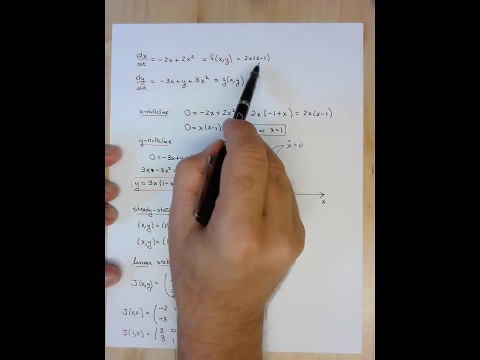 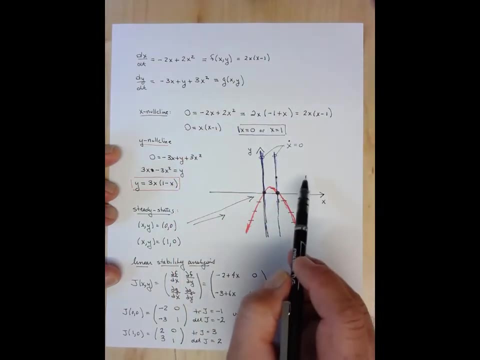 So if x is very large, it's greater than negative 1.. It's greater And it's greater than 1, so we're over here Right. Both of these terms- 2x and x minus 1, will be positive and the rate of change of x will be positive. 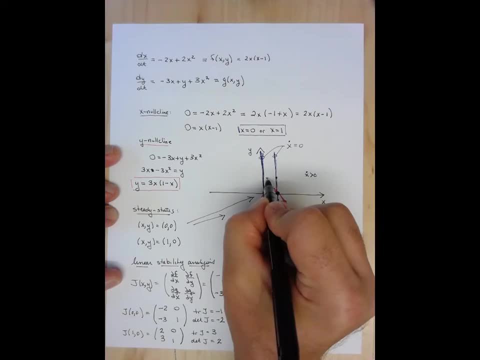 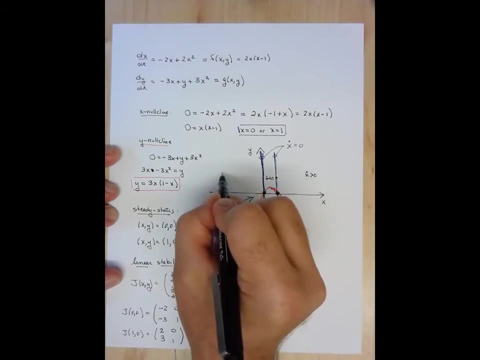 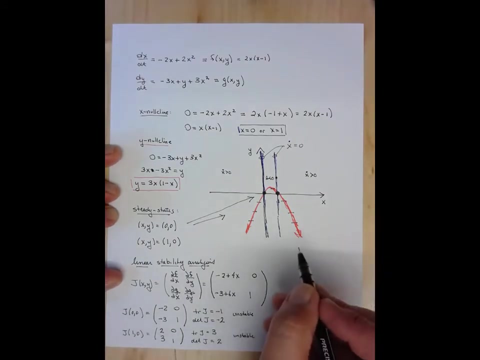 Now, when x is between 1 and 0, the rate of change of x will be negative, And when x is between is less than 0, the rate of change of x will be positive. The y-null climb also separates the phase space into two domains. 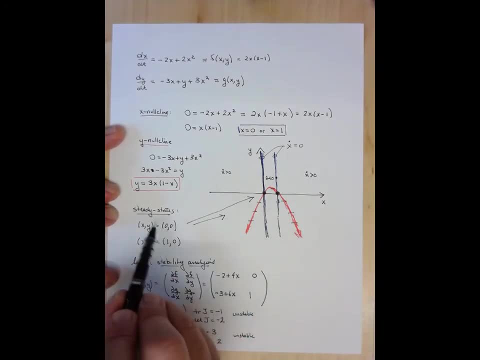 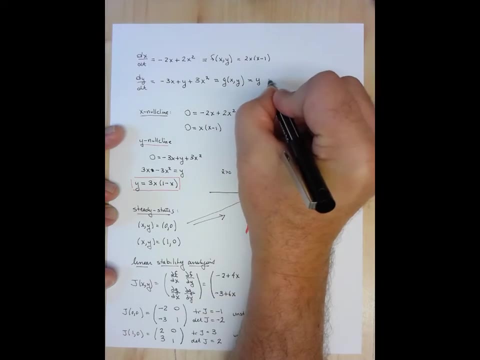 where the rate of change of y is increasing in one and decreasing in the other. When Let's see, if we look up here, we can write the right-hand side as y minus 3x times 1 minus x, And this means that if y is greater than 3x times 1 minus x, meaning we're above the parabola. 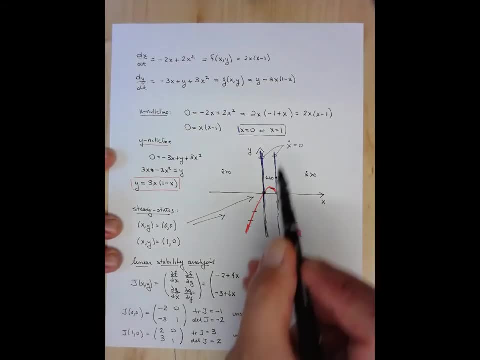 the rate of change of y will be positive, And if y is less than 3x times 1 minus x, the rate of change of y will be negative. So up here, above the parabola, the rate of change of y is positive. 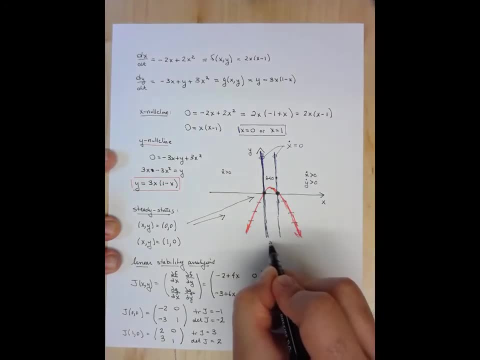 And below the parabola, the rate of change of y is negative. So we could indicate the direction of movement in all of these different regions In the following way: One thing we can do is actually put arrows on the lines crossing the y-null climb. 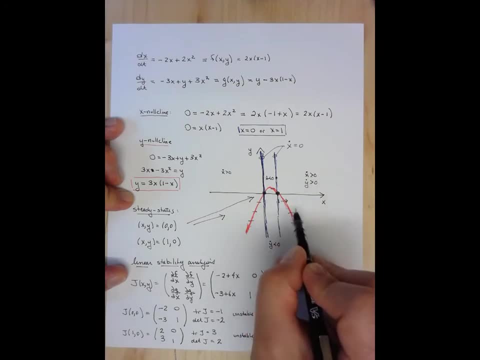 In this region, the rate of change of x is positive, so the arrows should be pointing to the right. In this region, the rate of change of x is negative, so the arrow goes to the left And it's positive again here. 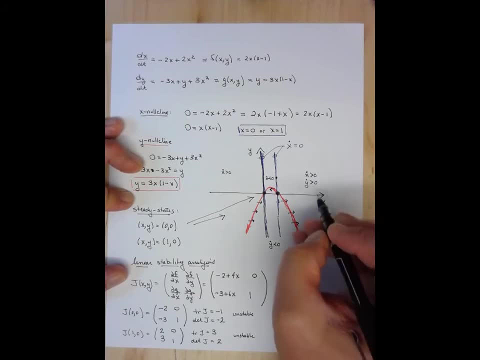 And now these arrows won't represent solutions. but In this region the rate of change of x is negative, so the arrow goes to the left. In this region, the rate of change of x is positive and the rate of change of y is positive. 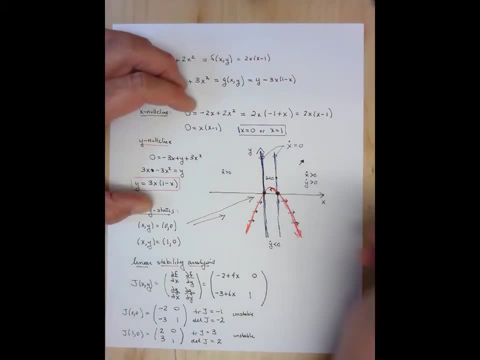 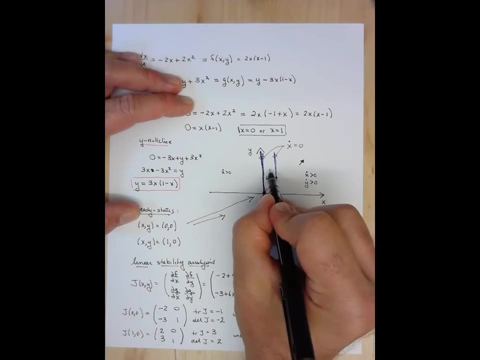 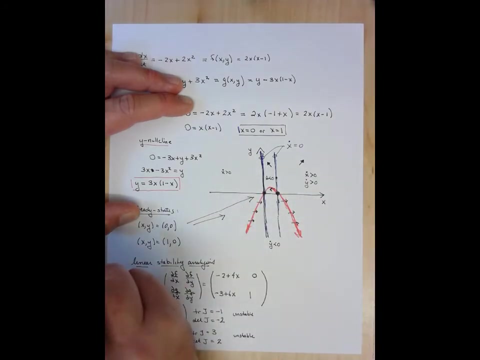 That would be indicated by an arrow going to the northeast. Here the rate of change of x has shifted, but y is still increasing, so it goes to the northwest, And here it should point to the northeast again. What about Down here? 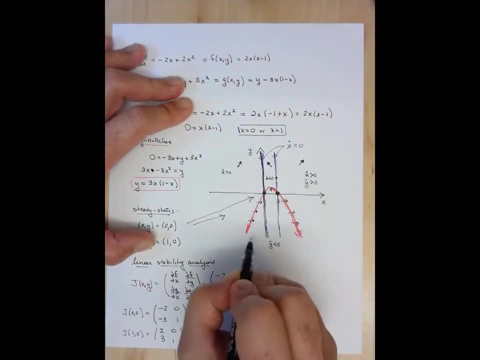 So when we move from this domain to this, the sign of the rate of change of y changes, so this will now be pointing to the southeast, Southwest And southeast And southeast. This region is the same as this one, so it's also. 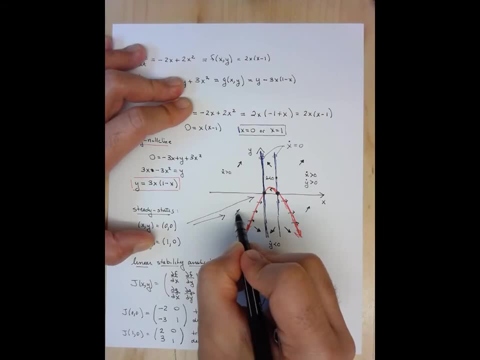 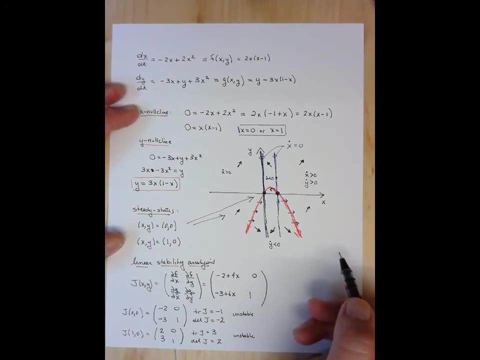 Moving in that direction. This region is the same as this one, Meaning there's no null climb that separated those two regions of the plane. So that's pretty good. We know that both of these equilibrium are unstable. Both the equilibrium are unstable. 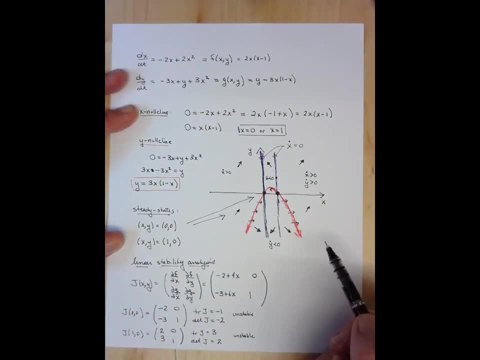 We've got a lot of information about the direction of the flow in the phase plane And We can see Just sort of think about what's going on near the steady states And see if we can get a little more of a sense of what's happening. 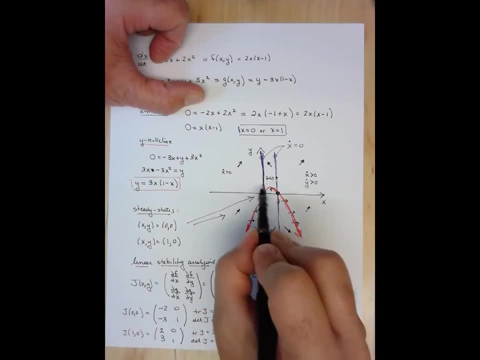 So, for example, if I was on, If I was on this point here, on the x-null climb, the rate of change of x is zero, but we're also in a region where the rate of change of y is positive. So there is a solution that goes vertically in this direction. 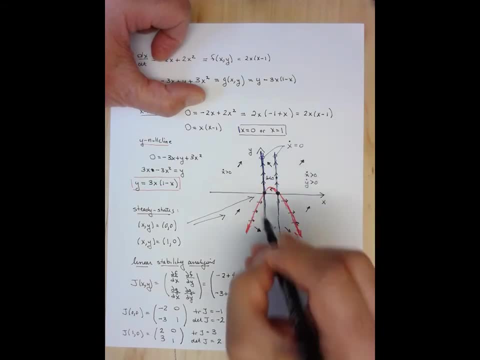 Here and here, And there's a solution that goes down in this direction. Now, how do I know that Anywhere on this null climb, the rate of change of x is zero And I've already determined the rate of change of y? 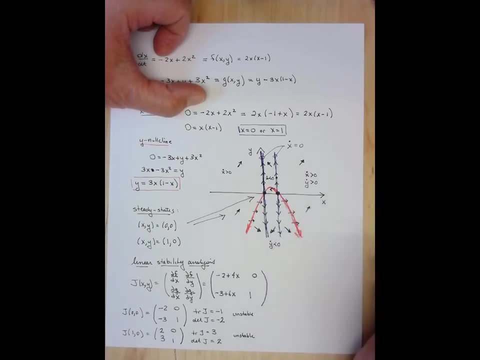 So I'm on the null climb, I'm going to stay on the null climb And I know whether I move up or down. So if you just sort of look closely at this equilibrium point in this region near the direction of flow is away in that direction to the northwest. 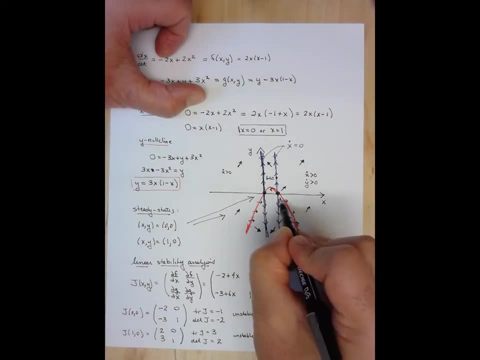 And in this region the direction of flow is to the, To the. Sorry, this is northeast, The direction of flow here is southeast, The direction of flow here is southwest And the direction of flow here is northwest. So that sure does look like it's going to be a node. 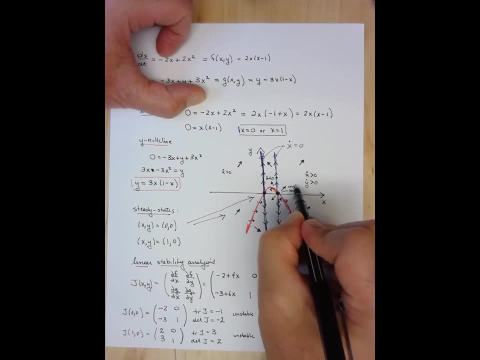 We already know it was unstable. So it's an unstable node, And this one. if I do the same thing and think about what's happening nearby, the flow is moving to the northeast over here. It's moving to the southwest in this region. 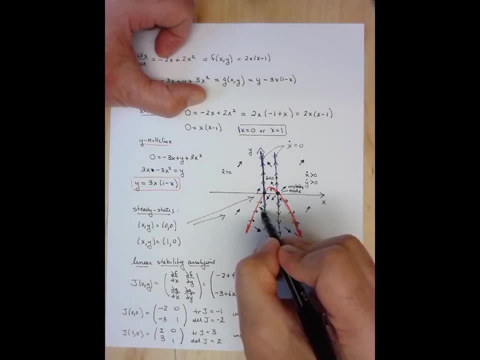 And this region is moving in that direction- southeast, And in this region up here it's moving northwest. So when I look at these flows, this looks very much to me like a saddle, Because if a solution was moving in this direction, 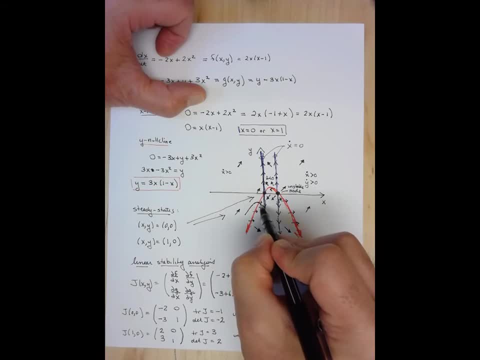 and then, crossing the null, climb in that direction and then it would have to move down and then it would asymptotically approach that axis. If the solution actually crossed this null, climb in this direction, it would then move to the east upwards, like that. So you see how it looks like. there's just some indication. 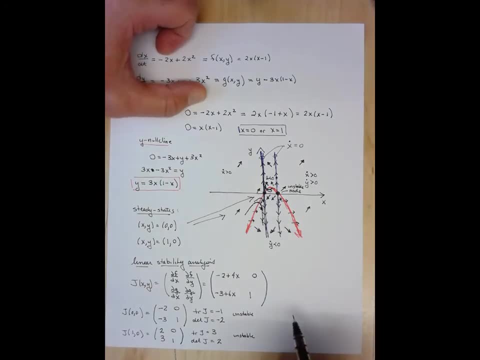 here that this is going to be a saddle. Saddles are unstable, which is consistent with what we have here, So I'm thinking that this is going to be an unstable node and that this will be sorry. 0, 0 is the saddle, So this is a saddle. 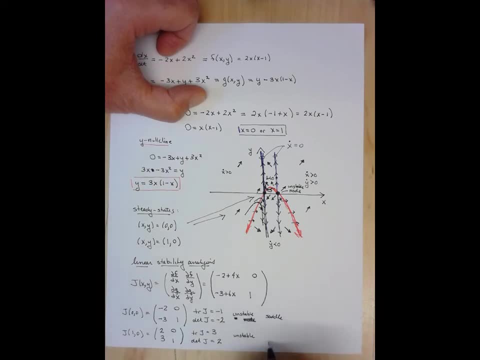 and this is a node, and I can confirm this algebraically by considering the eigenvalues of the Jacobian matrix of this. So in the, in the to find, to figure out what those eigenvalues are, remember that an eigenvalue is going to be the opposite of the trace of the Jacobian plus or minus. 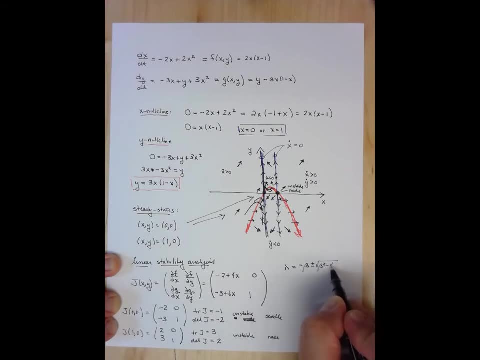 the square root of the square of the trace minus 4 times the determinant divided by 2.. We haven't discussed this in class yet, but this is the the solutions of what are called the characteristic equation of the 2 by 2 matrix, when we're solving an eigenvector, eigenvalue. 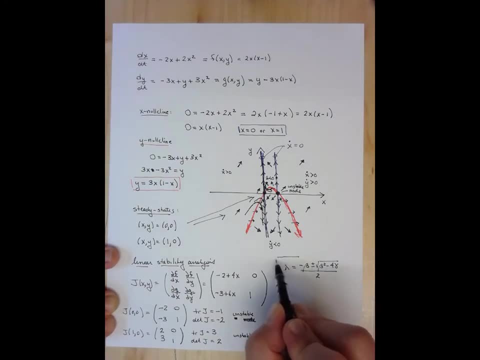 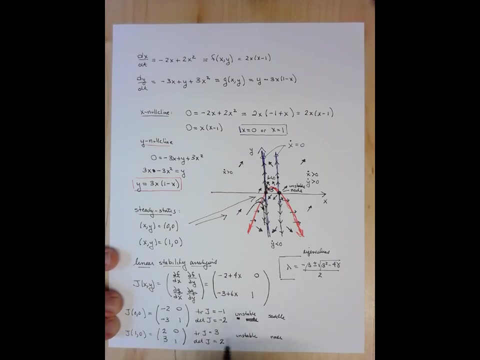 problem. If you just take it as a given that this is a formula for the eigenvalues of these constant coefficient 2 by 2 matrices that we see here and do a little substitutions, several substitutions, you'll find that I did this in advance actually. 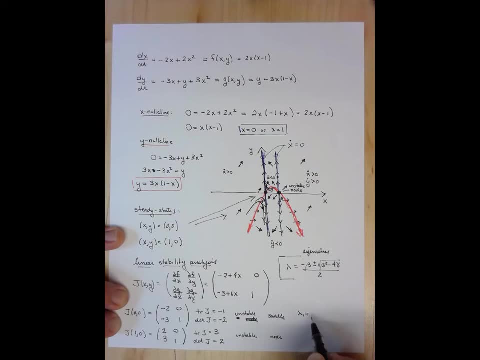 so one of the eigenvalues in this case is negative- 2, and another one is 1.. So these are real numbers, and one's positive and the other is negative. It corresponds to a saddle. In this case, one of the eigenvalues is 2, positive 2, and the other eigenvalue is positive. 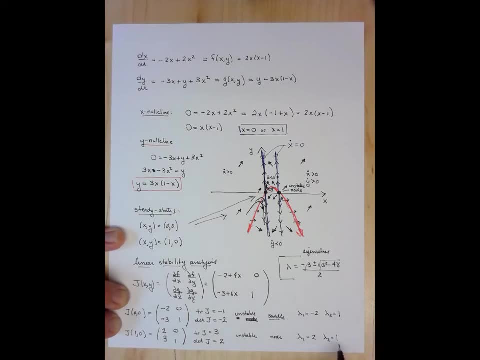 1.. So these are real and distinct eigenvalues that are both positive and that corresponds to the unstable node, And you can check my work here. You can let me just do one of these. One of the eigenvalues was negative- 2 here- and one is 1.. 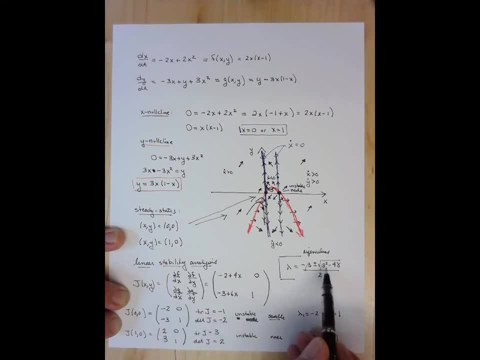 So if I were to do this again- I'm going to do this again- If I, the beta is the trace of the Jacobian. so if I take negative 1 for beta and if gamma is actually negative 2, then this will be negative 1 squared, which is 1 minus 4 times.